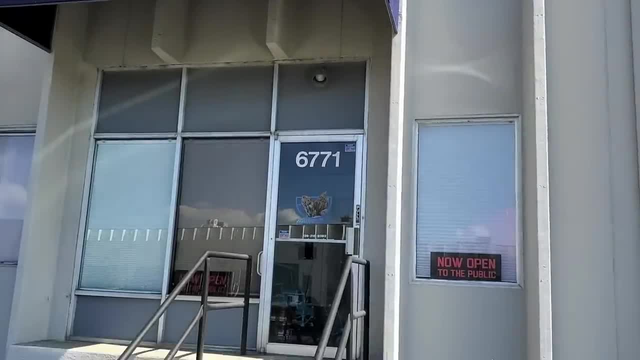 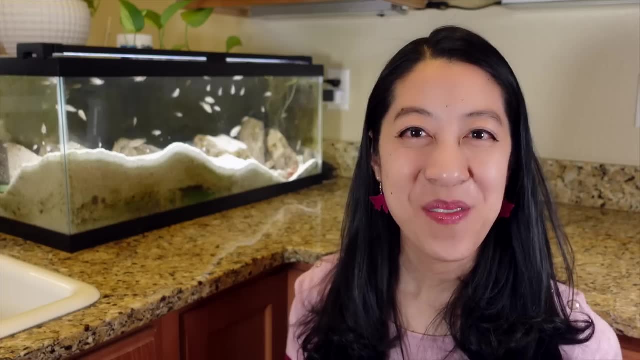 store and visit their warehouse in person if you want to. They're located in Commerce City, Colorado, among a lot of other warehouses, So you basically go there and you go. am I in the right place? But when you enter in, first thing you see is a ton of different kinds. 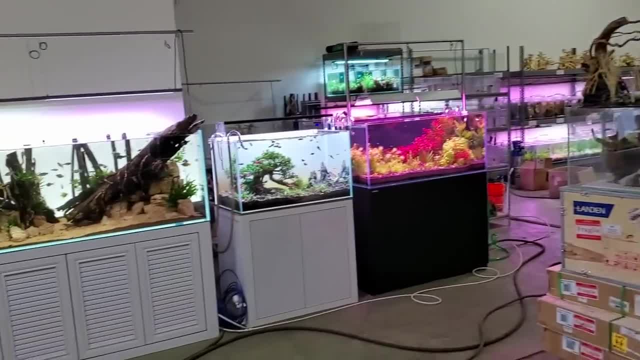 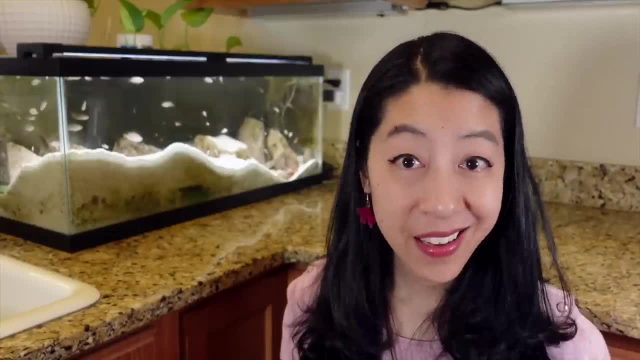 of aquascapes like totally beautiful, You're allowed to take pictures and film in there. The owner, Tommy, greeted me and he was like, yeah, you can film everything except for my competition tank that he's doing for some kind of aquascaping contest. 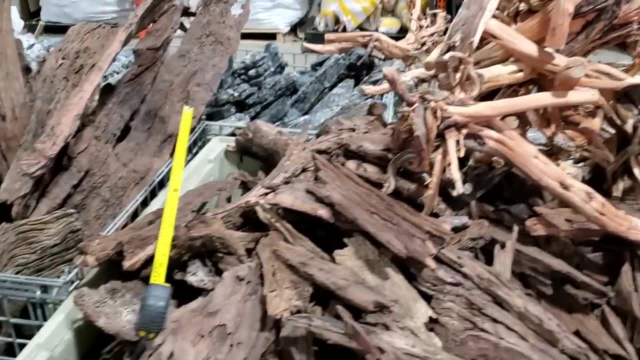 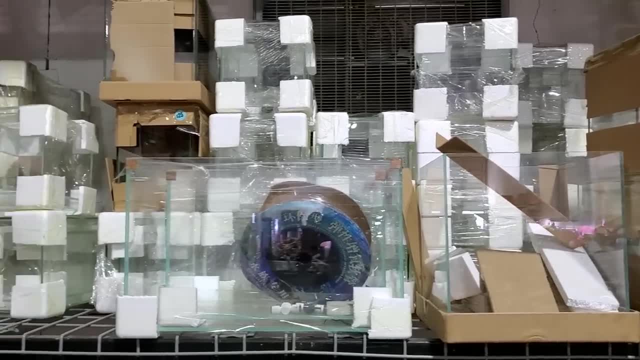 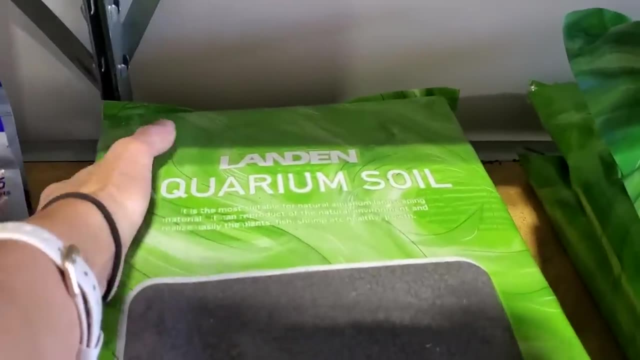 So that was really cool. Obviously, there's bins and bins of hardscape, you know rocks, driftwood, stacks of rimless tanks and every kind of you know aquascaping supply that you could think of, including the active substrate I was looking for, Since I didn't know what I was. 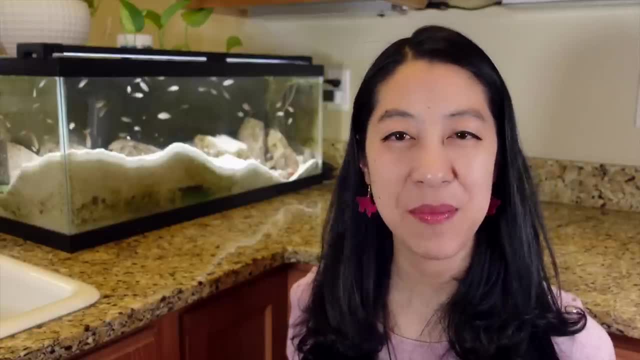 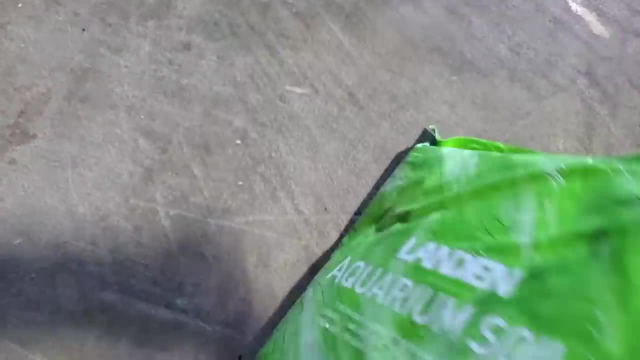 doing. you know I'm not an aquascaper. I asked Tommy- I think that's his name, the owner- what does he recommend? And he said: well, if you don't care about getting the name brand stuff, he personally uses Landon. 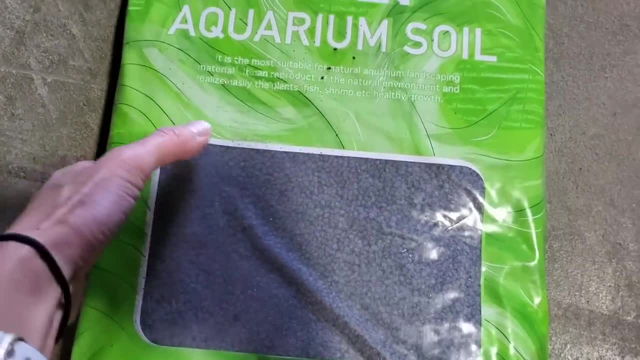 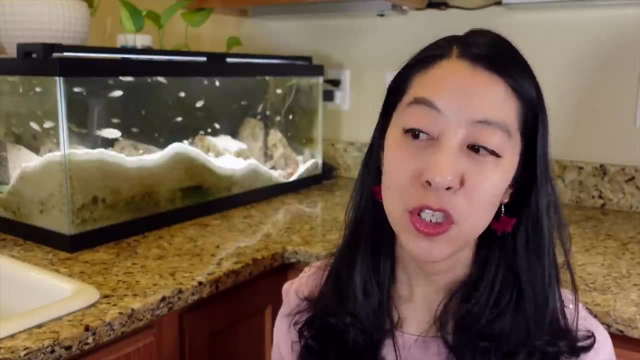 In all of his aquascapes because he feels like it's good quality stuff but it's a lot more cost effective and affordable. And, yeah, that's what I ended up getting. I also, you know, with so many aquascapes in that warehouse to maintain, I asked him. 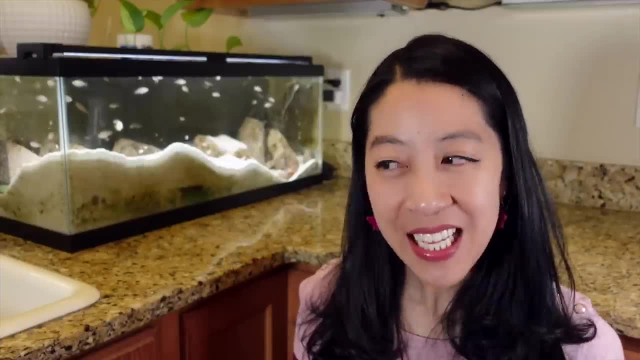 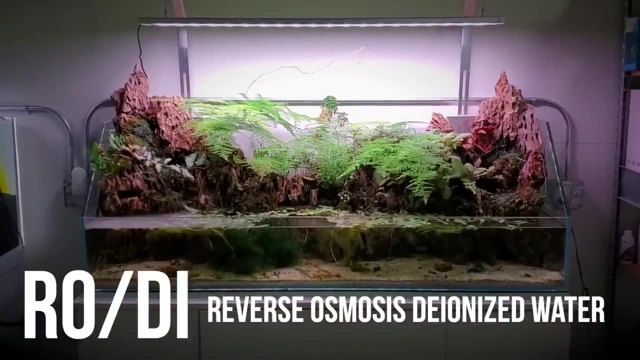 what is his secret to having algae free tanks? And he says- and this is not the first time I've heard this- actually He says he uses RODI water, So reverse osmosis, deionized water, it's stripped of everything And then he remineralizes. 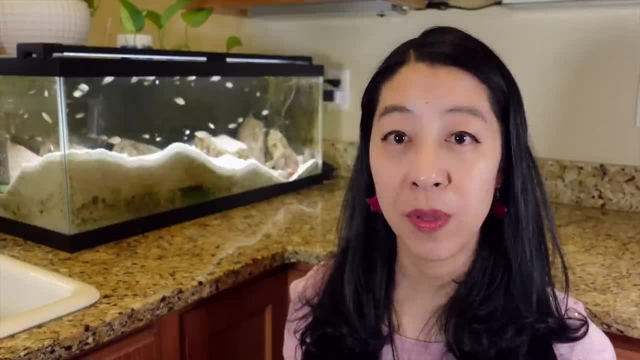 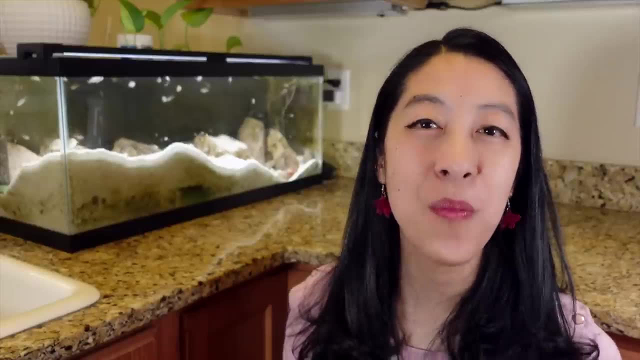 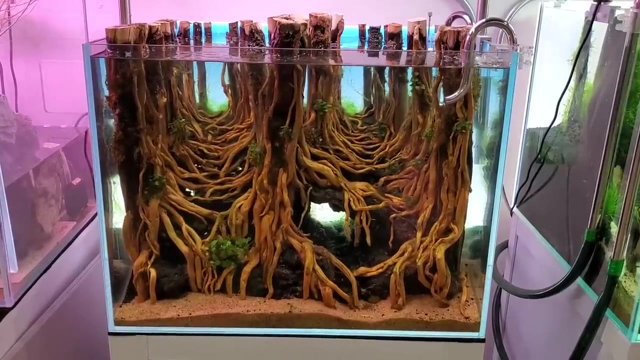 or re-doses in plant fertilizer and minerals for the plants, And that's how he's able to keep them algae free. I personally do not have the time for this, So, but I figured I'd pass along the advice to you if you want to try it. There was this hardscape looking forest where it was only driftwood. 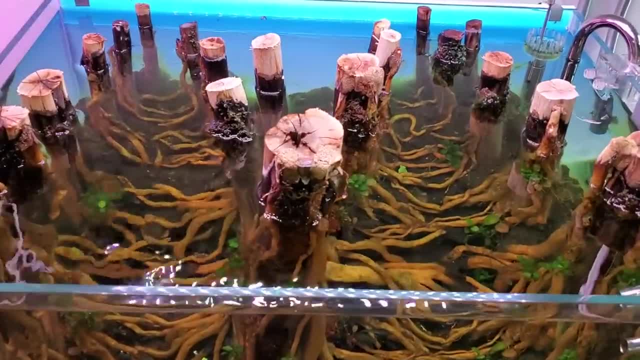 It looked like tree trunks with roots down. Not a lot of plants in there, but there was one single pea puffer swimming around among all the trees. And it looked like a tree trunk with roots down. Not a lot of plants in there, but there was one single pea puffer swimming around among all the trees. 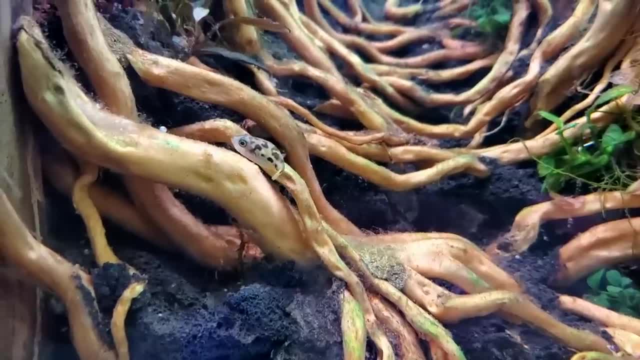 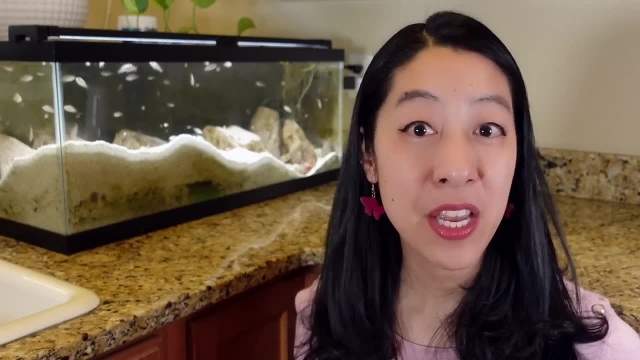 And so I thought it was really, really cool. I saw that take and I was like I need to have this, especially with the pea puffer in it, So super adorable. It's a family-owned store company, So you know Tommy was there, his wife and baby. If you want to check their. 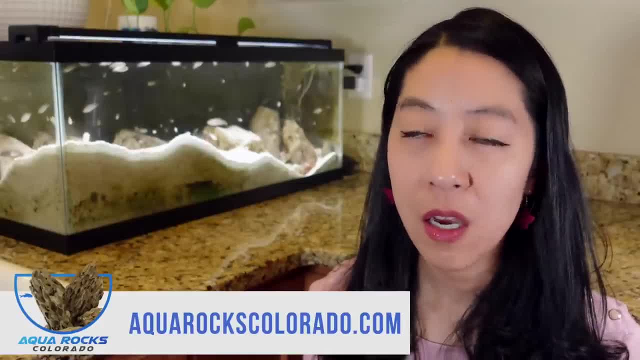 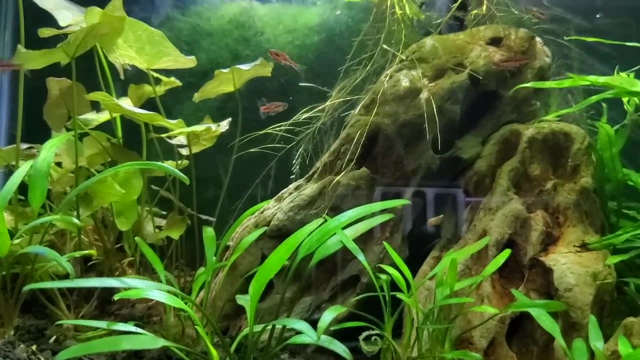 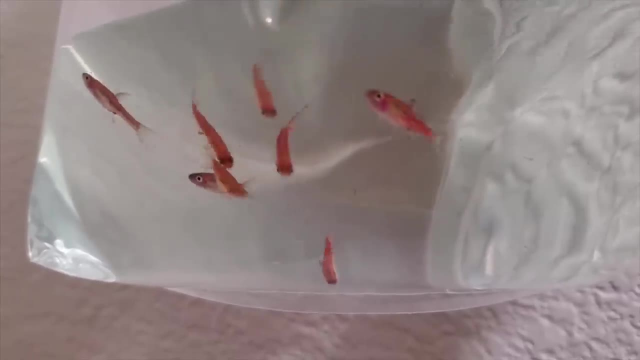 store out they are. I'll put the link in the description. I think it's aquarockscoloradocom- Now to do a big renovation of my aquarium. I basically waited until I had no animals, So it was right after I rehomed the chili rasparas And I was like, okay, now is the time. 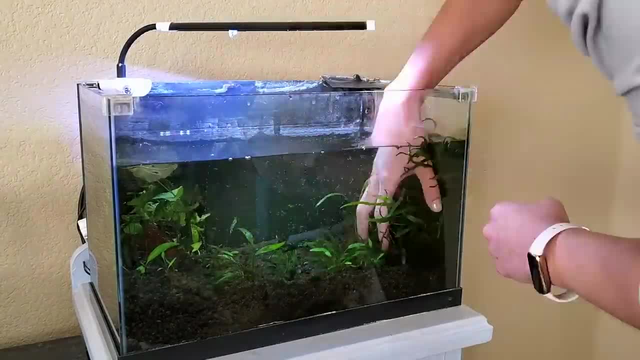 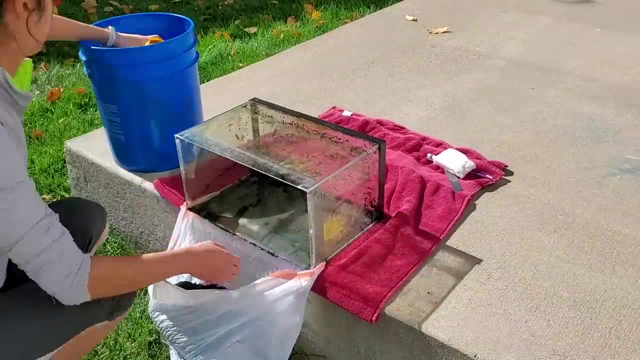 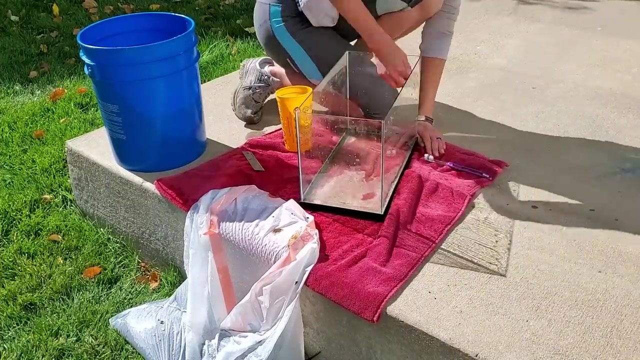 So I began the laborious task of, you know, removing all the plants, the equipment, draining all the water, taking the tank outside and removing all that stinky substrate which you know it's full of mold and rotting organics in there which are good for plants but it smells. 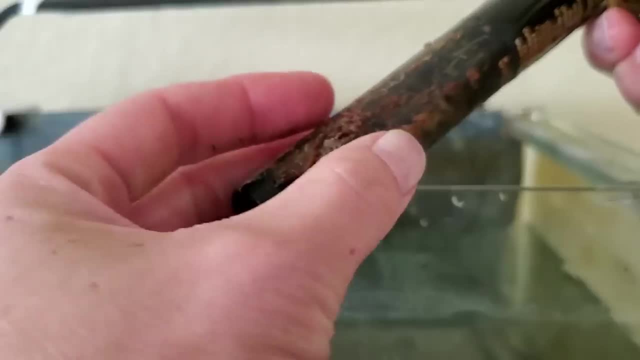 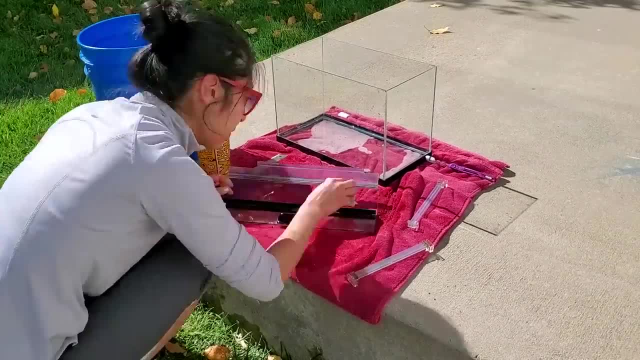 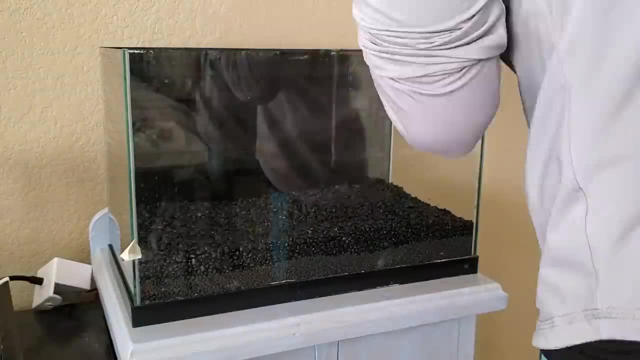 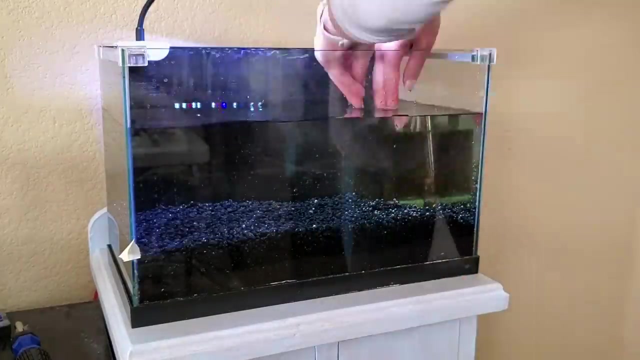 the algae and gunk that I have neglected over the months. Then I brought the tank back inside and I decided to put one and a half inches of the land and Aqua soil at the very bottom, And then I capped it off with one and a half inches of just regular black aquarium gravel. 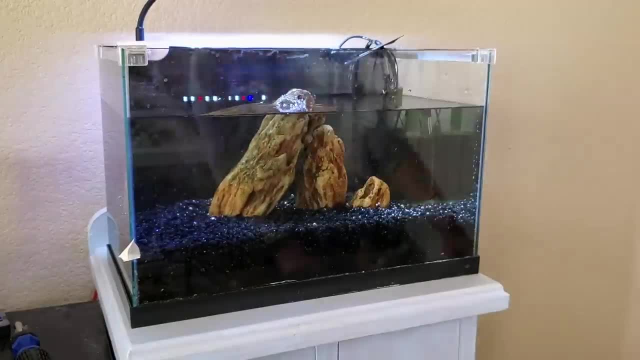 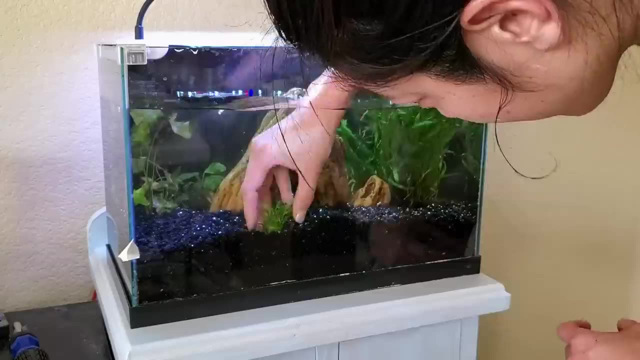 that I probably got from Petco. Then you just replant everything back the way it was. So I have my dragon stone thingy in the middle. We've got the narrow leaf Java fern on the right side, the dwarf aquarium lily on the 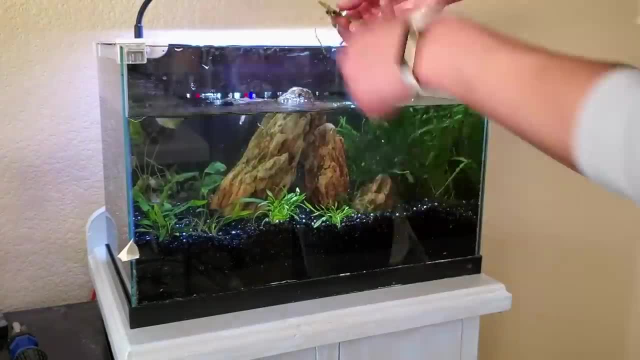 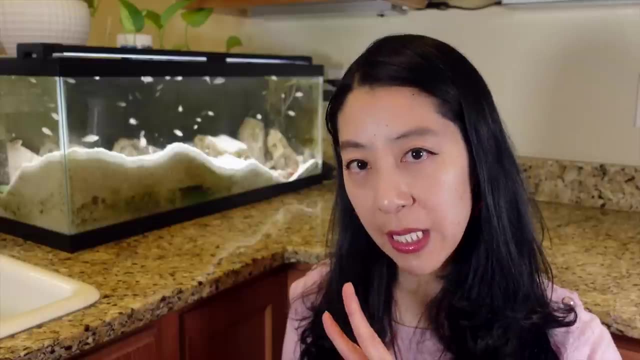 left side, lots of cryptocoryne plants in the front, And then I have a floating corral of salvinia right in the middle, right over the hardscape, so that it won't grow algae. Two days later I noticed that the water was forming foaming bubbles, which usually means 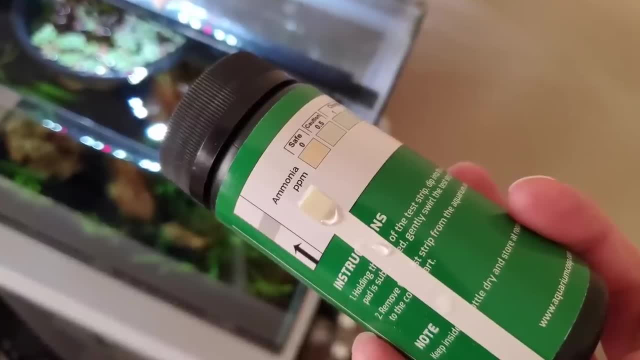 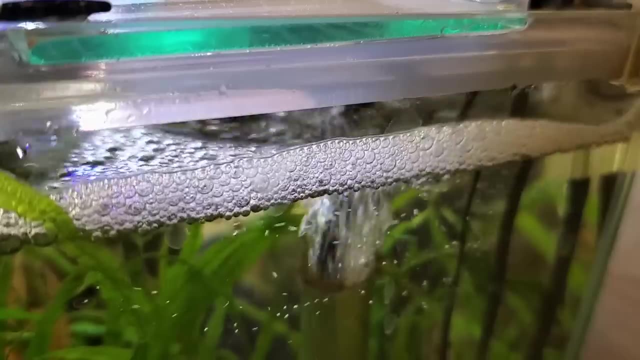 something's off with the water chemistry. So did some measurements. There's like a slight bit of ammonia, No nitrate, no nitrate. So you know, good thing I have no animals in there. Two weeks later the foaming was getting like even worse. 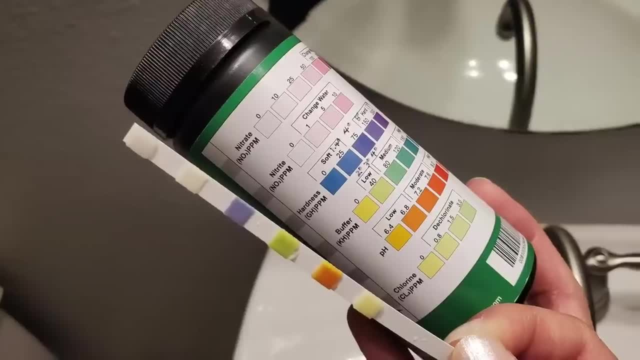 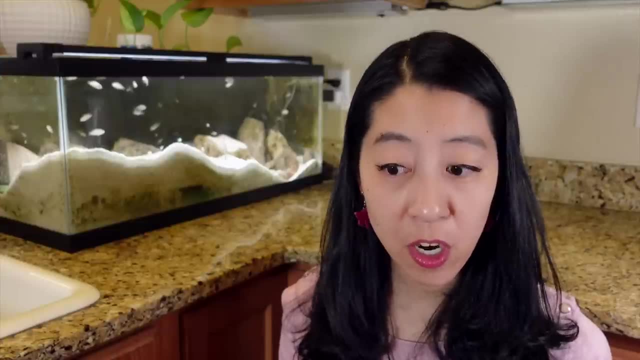 So same thing. little traces of ammonia, not so much of the other stuff. I think the combination of, you know, the Aqua soil was leaching lots of nutrients into the water. column, Plus the dwarf aquarium, lily and cryptocorynes were really unhappy with the having their 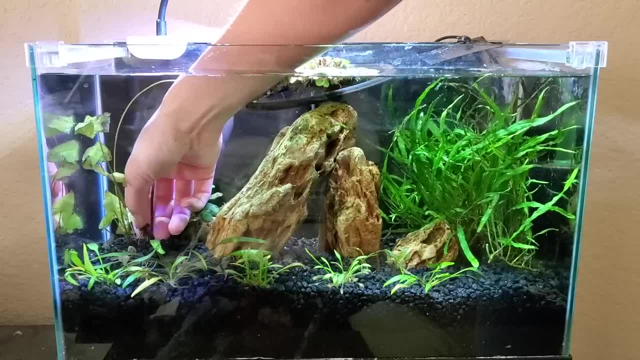 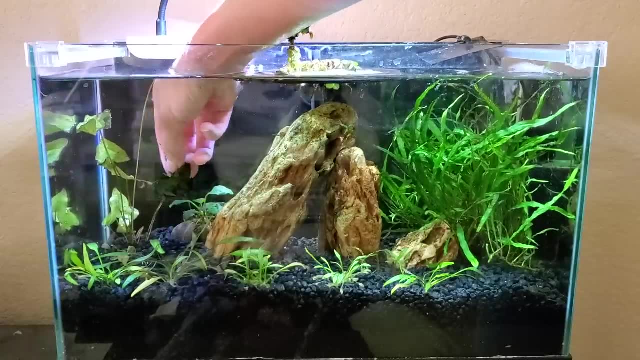 environment suddenly changed, So they started melting back and there was a lot of melted leaves, Yeah, And all these excess nutrients meant, yeah, there was some blue green algae or cyanobacteria that formed, And so I ended up having to do some maintenance to remove it and all of the melted leaves. 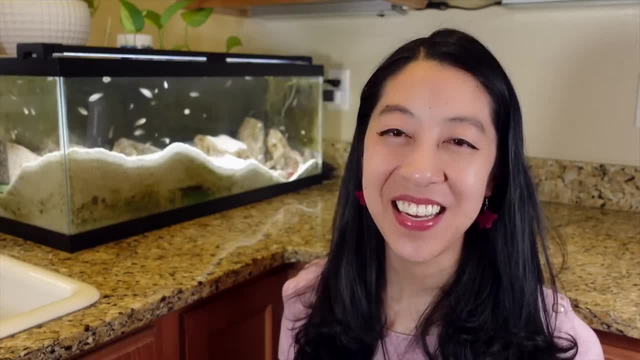 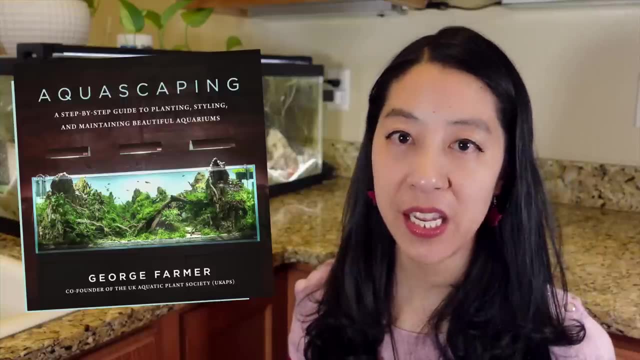 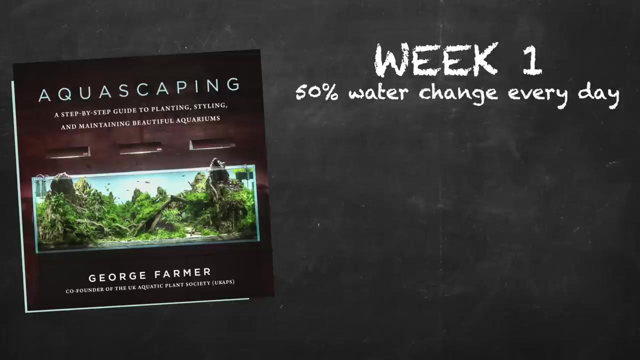 in the tank. What I probably should have done was- and I'm belatedly remembering this- George Farmer is a famous aquascaper and he recommends every time he sets up a new tank, especially if it has nutrient rich substrate. he always says in week one he does 50% water changes. 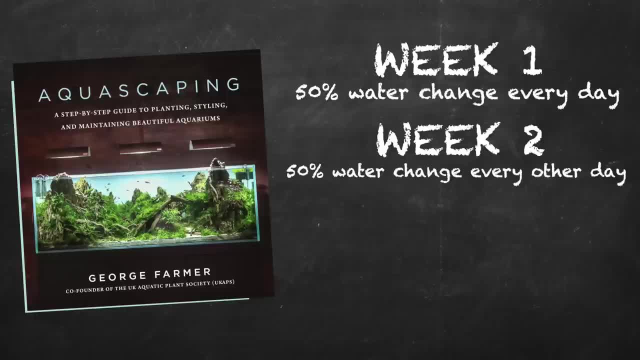 every single day. Then, week two, he does 50% water changes every other day. week three, he does water changes twice a week And then finally, week four, he's down to one water change once a week. And that is all to remove all those excess nutrients so that you won't develop those. 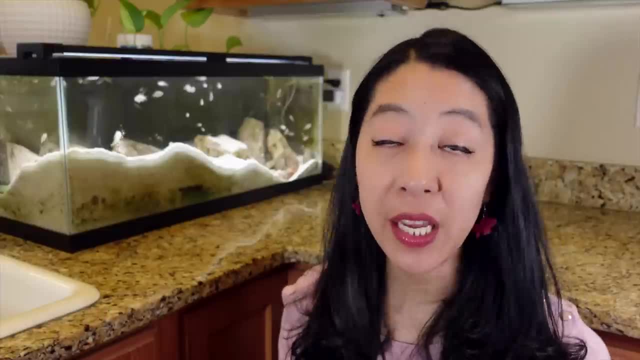 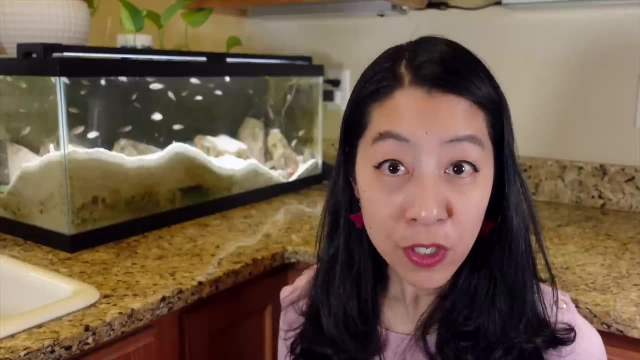 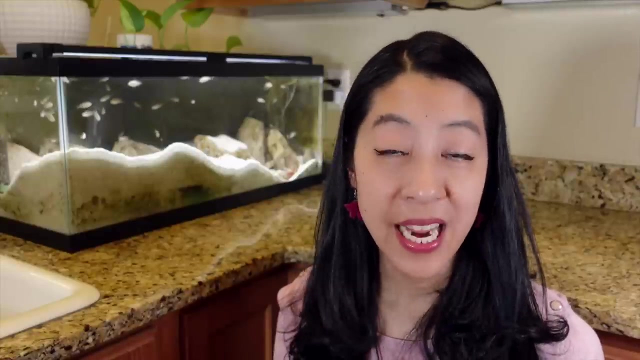 algae problems that I experienced Bottom line. good thing I did not have any animals when I first set up this tank, because active substrate will release a lot of nutrients at first and then slowly it'll kind of decrease over time. The plants and the bacteria will be able to absorb them as well and handle the increased. 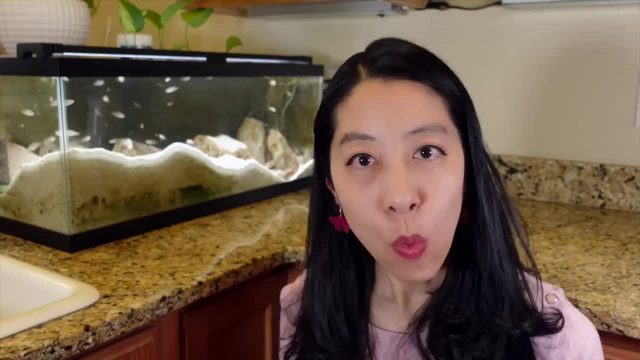 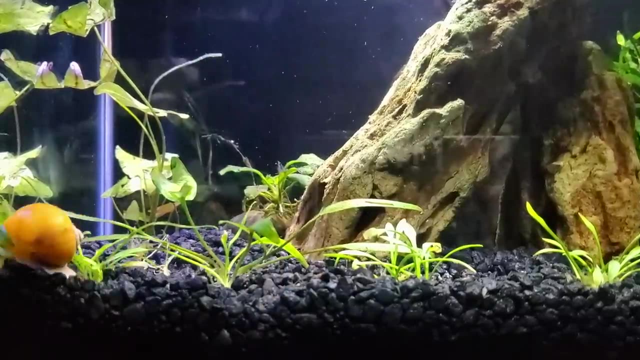 bio load and then it'll be safe to add your plants once your water parameters are looking good. Finally, the tank parameters got stable enough where it was safe enough to borrow Sunstreaker- the mystery snail for my 20 gallon- put him in the five gallon for a little while to eat. 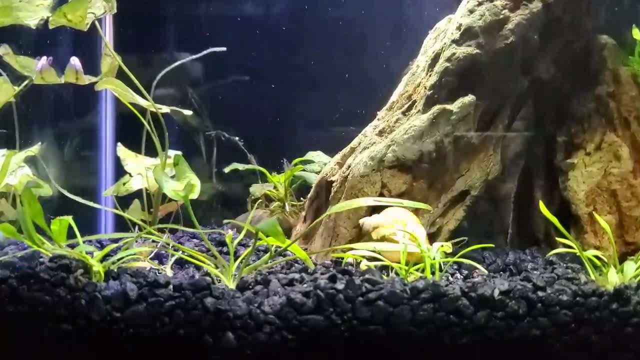 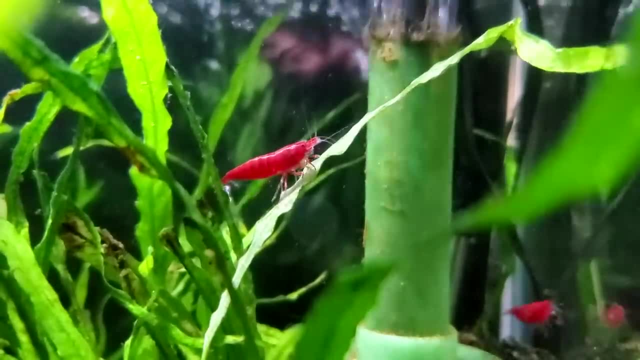 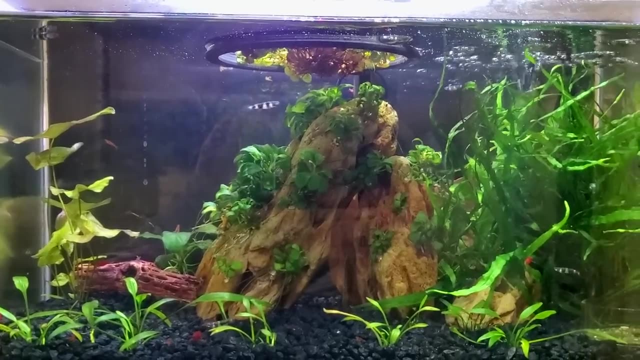 up all the melted crip leaves. He does a lot better job than I do anyways. And then the first animals I added were the neocaridina shrimp. I got the bloody Mary shrimp- It's a type of cherry shrimp, I guess you could say- as well as clown killifish and everything was going well, and hunky dory. 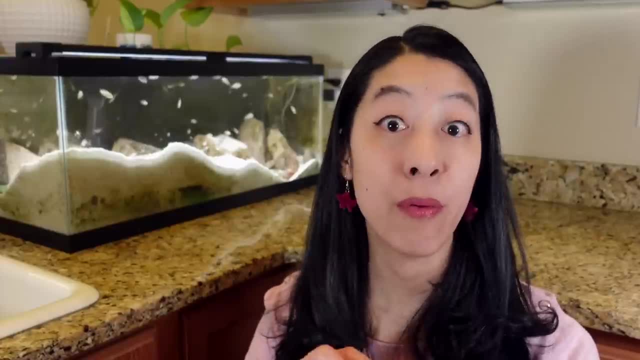 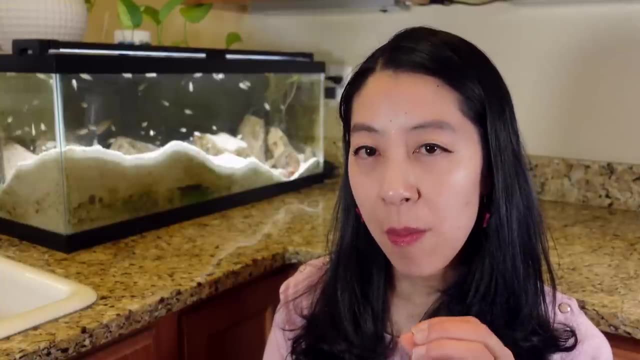 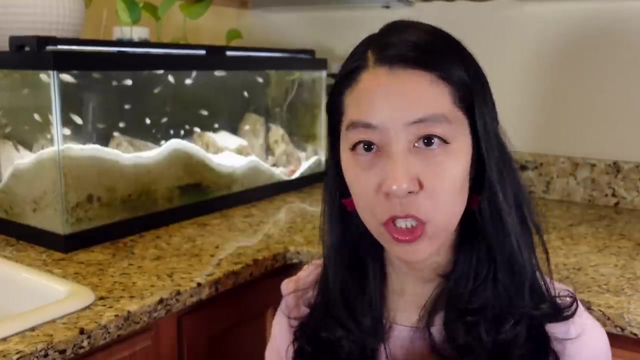 The plant stopped melting, I think. eventually their roots got deep enough where they were reaching the Aqua soil. But then about, I would say, three months in, I saw my first shrimp death and I was like what's going on? So you know, when an animal dies, first thing you do is do a water test. 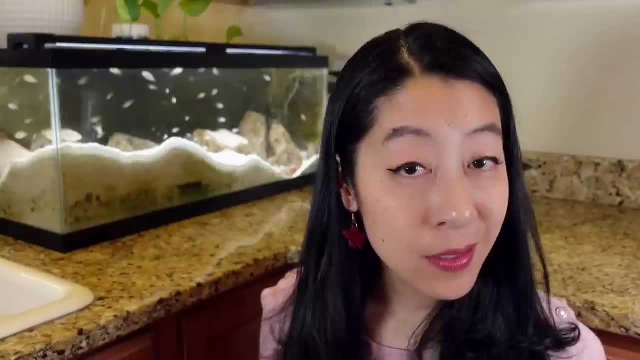 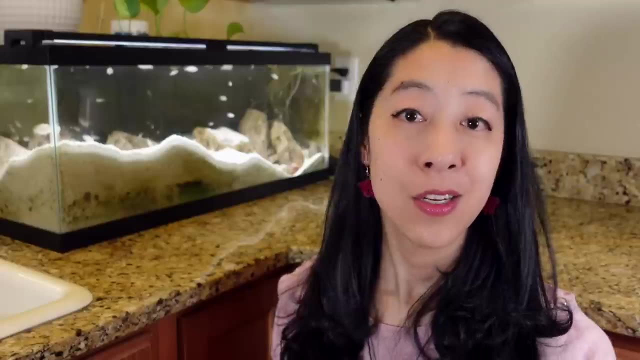 I hadn't been doing. you know again: myeloma, No maintenance, Aquarium keeping. lifestyle is to not do a ton of water changes because I use aquarium plants to consume all the excess nitrogen in the tank. Unfortunately, the nitrogen was not the problem. 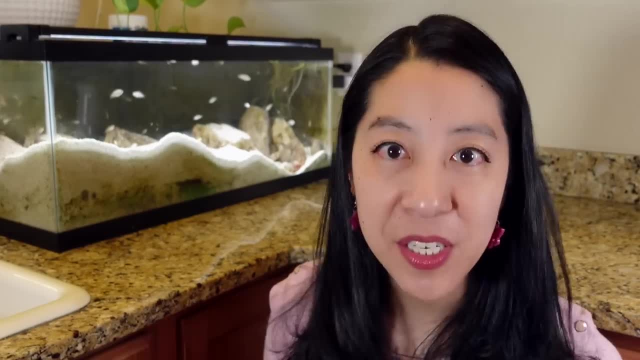 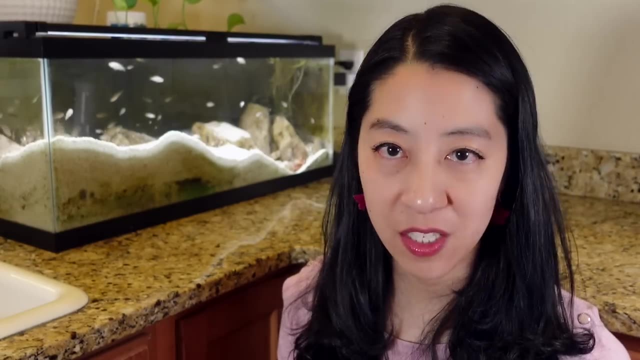 It was actually the pH, GH and KH had just like plummeted over time, which I guess is to be expected with Aqua soils, because they have these buffering qualities to them. That's why they're also called active substrates, because they will change your water chemistry. 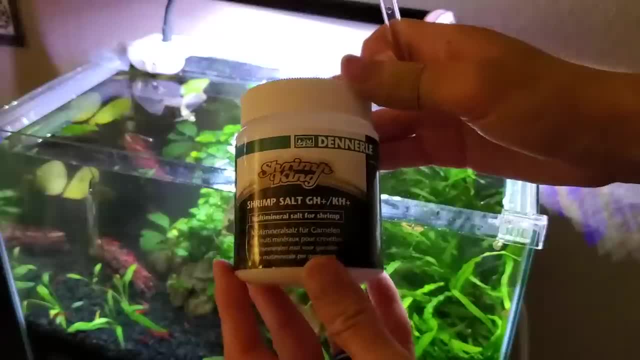 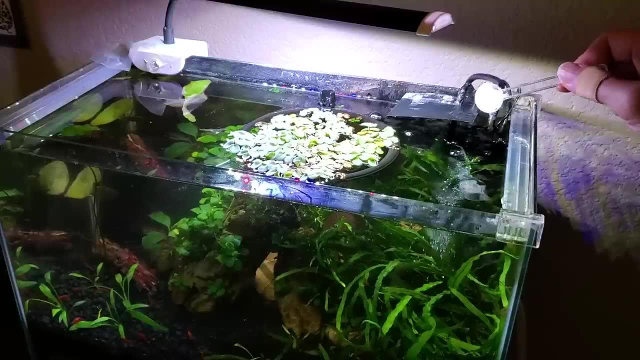 parameters. So I freaked out, did a water change and I bought Dennerle Shrimp King shrimp salt, the GH plus, KH plus kind, which is for Neo-Cardinia species, as well as Aqua vitro shrimp exo- I think is what it's called. 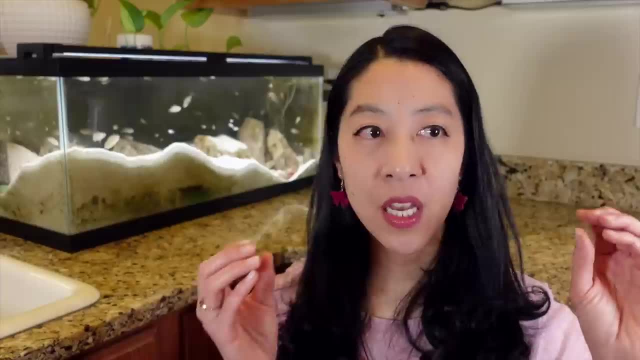 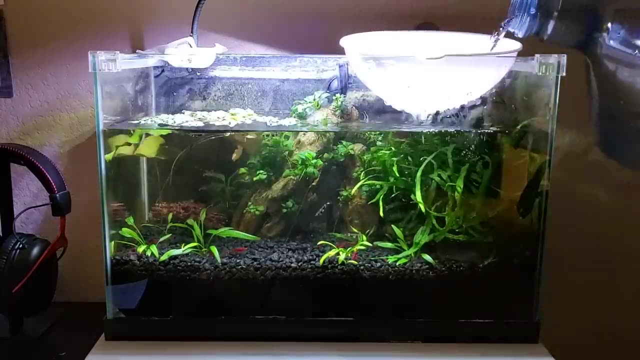 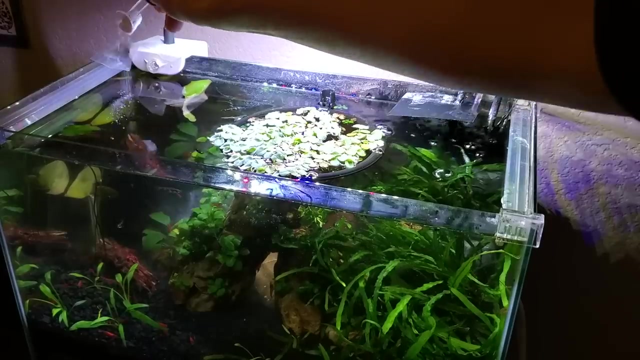 And that's extra iodine again to help with molting. because my guess was, because of those low water chemistry parameters the shrimp were dying from failed molts. Unfortunately, the only way I could Keep them alive was to have to do at least weekly water changes and then weekly dosing. 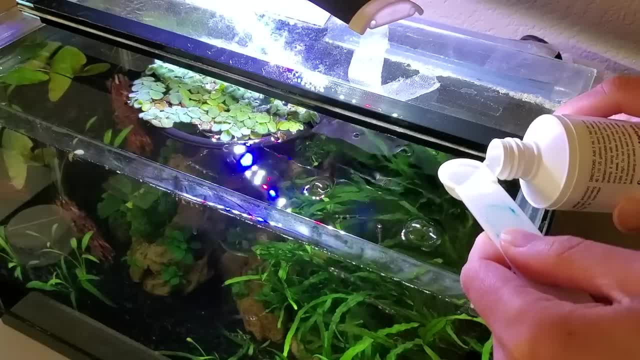 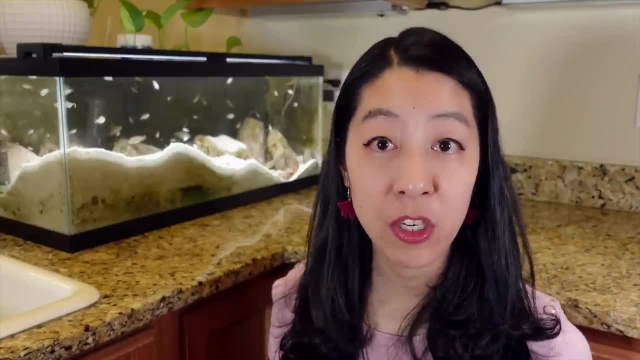 of the shrimp, salt, minerals and the iodine, And then I don't know what was going on, but the pH, GH and KH were all higher and at what I would consider good amounts for cherry shrimp, but I was still getting shrimp deaths. 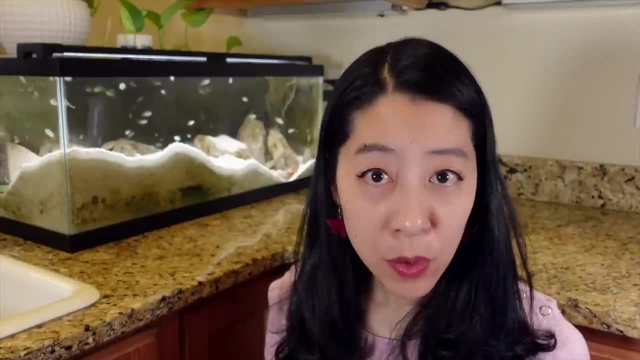 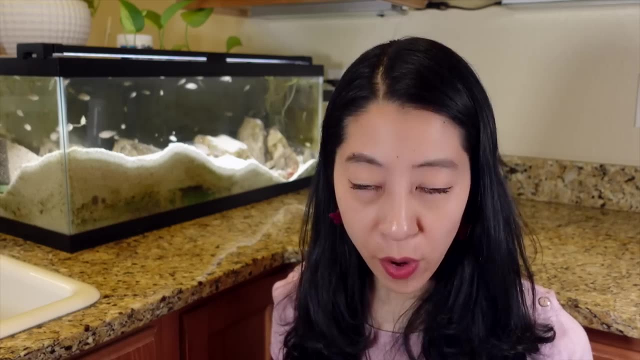 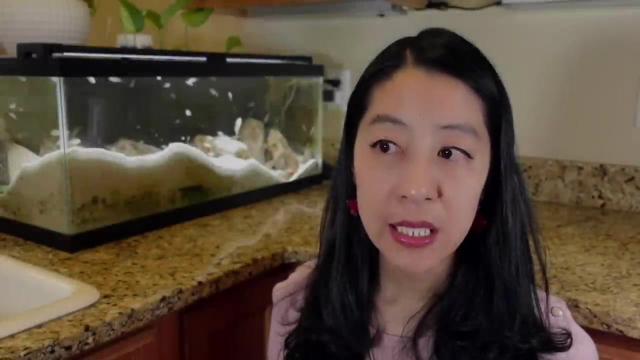 So I'm not sure if it was like the iodine amount wasn't enough. but then I looked online and there weren't Really any good iodine tests for freshwater aquariums Like. the reviews I saw on Amazon were just abysmal, honestly. the constant one-off deaths. here and there, and the constant water changes were really taking a toll on me. It was just so stressful trying to keep on top of water chemistry all the time because of this Aqua soil that I put into the system. Okay, Okay, After, I would say, a month of failing to consistently prevent shrimp deaths, it was just time to. 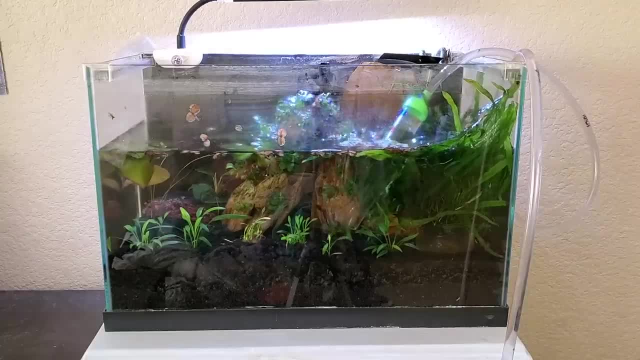 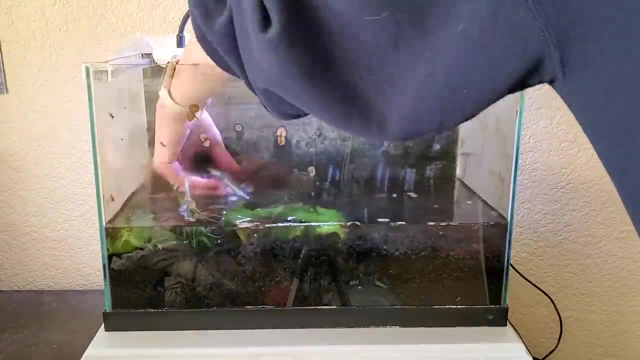 throw in the towel. I was now going to have to redo the whole tank again, get rid of that Aqua soil, And this time I'm going with a completely inert substrate. I'm done, I'm just going to go with good old Petco black aquarium gravel. 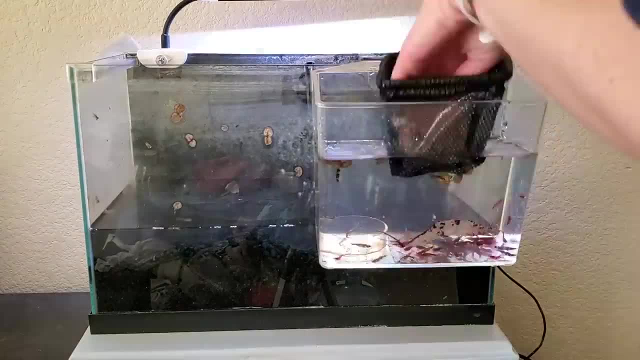 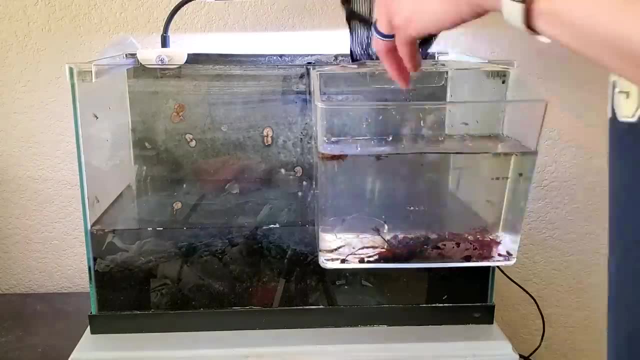 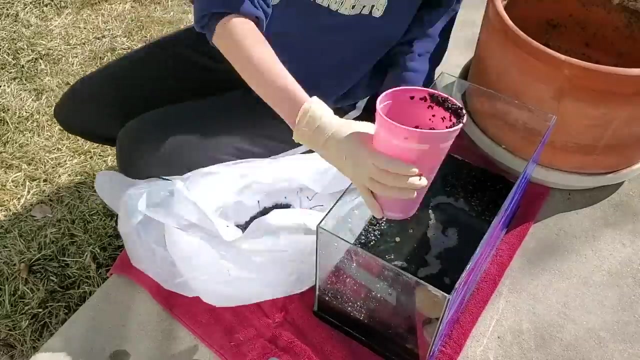 The tanks. tear down is the same process before, but this time I have animals to deal with, So great. Drain the water, remove the plants and the equipment and then just sit there with my little net, picking out one shrimp or one killi fish at a time. 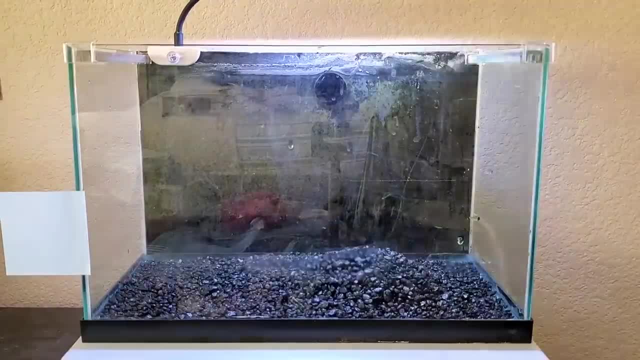 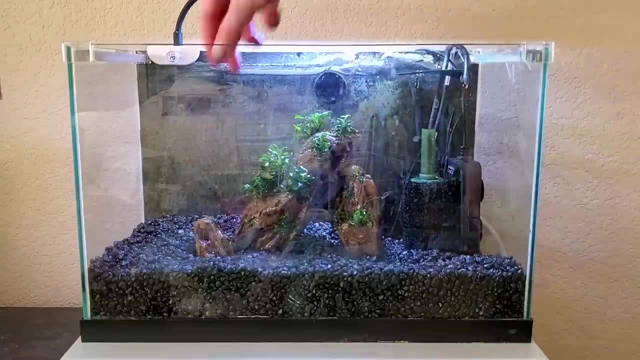 It took a long time, to say the least. Now, since there are zero nutrients in that gravel, I put a ton of root tabs exactly where I knew the cryptocorynes and the dwarf aquarium lily were going to be, as well as my water. 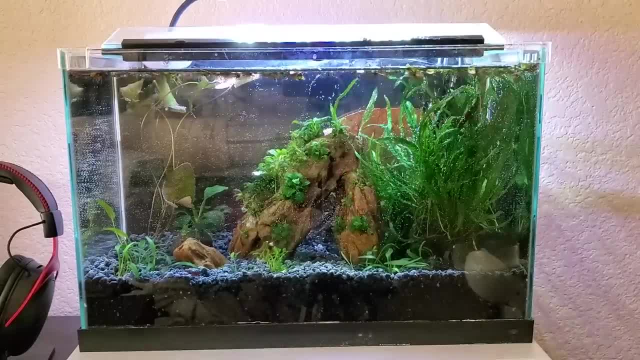 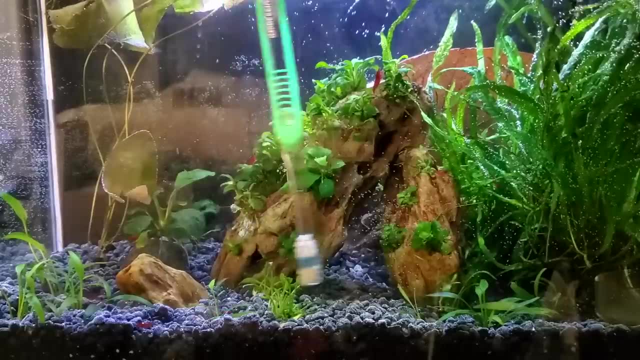 is actually on the soft side, So I did end up dosing One teaspoon of shrimp salt as well as one teaspoon of the iodine. You can see a ton of micro bubbles all over the tank, because I'm doing this when it's 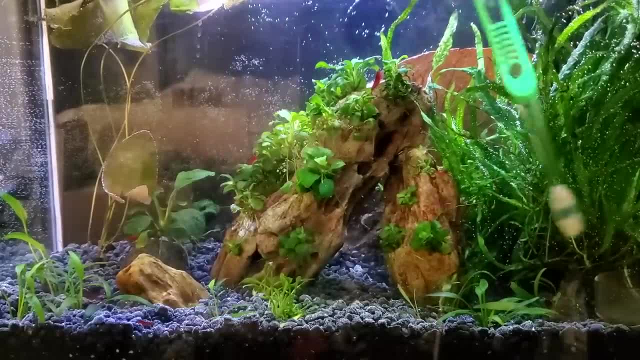 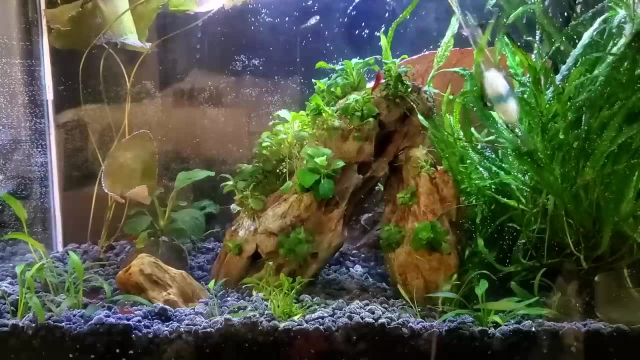 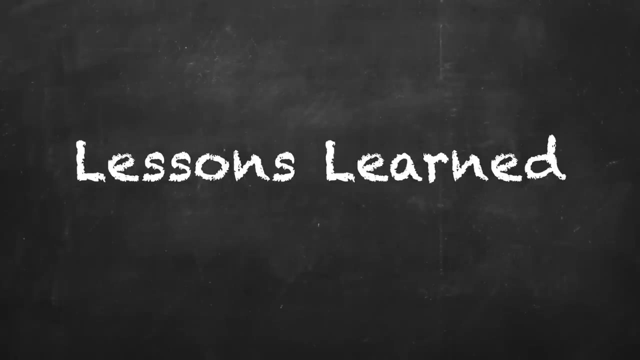 winter There's- it's pretty chilly- groundwater out there coming out from my tap, And then when you warm it up, the excess oxygen in the cold water can no longer be held in the warmer water, So then it just gets out, gassed into actual bubbles, into the tank. a lot of fun. 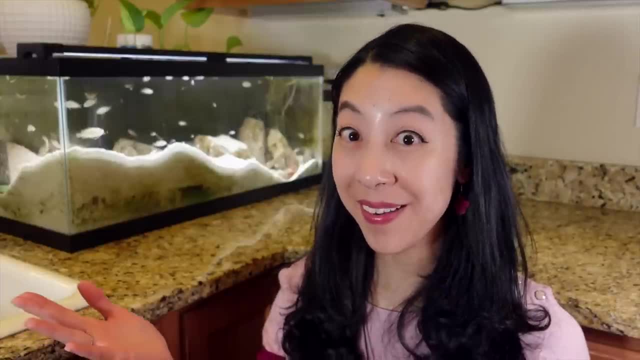 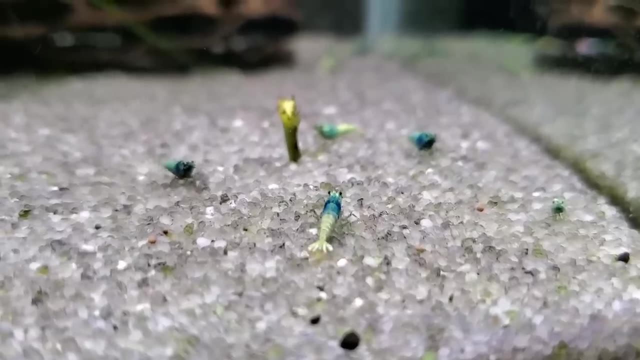 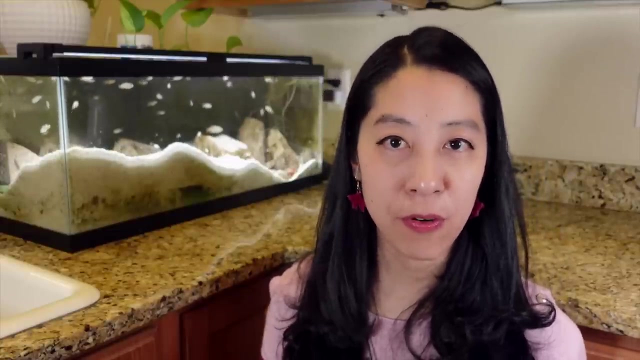 Now some of you clever folks out there may be thinking: Irene, this was your chance to get your dream shrimp, those Caridinia blue vault shrimp. Why didn't you do that? I mean, they do like soft acidic water, but the fact is, active substrates only buffer. 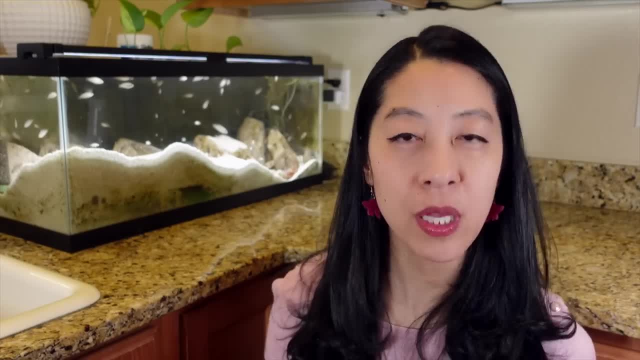 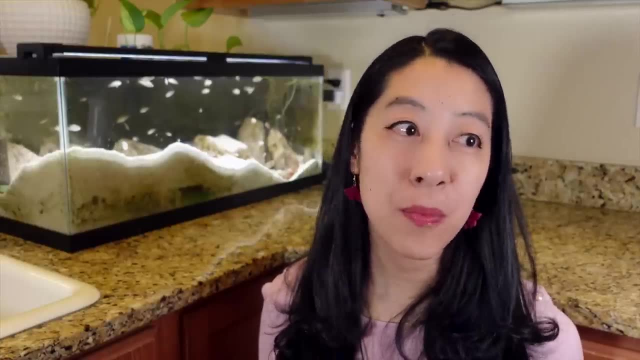 or change your water parameters for about a year or two, Like people try to extend it by using RODI water. I'm not about that life, obviously, So I would probably be having to change my active substrate every single year And 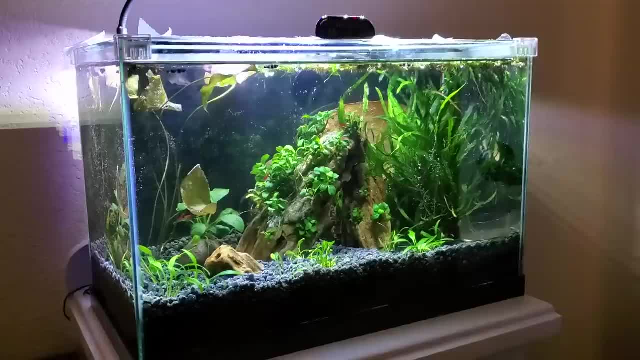 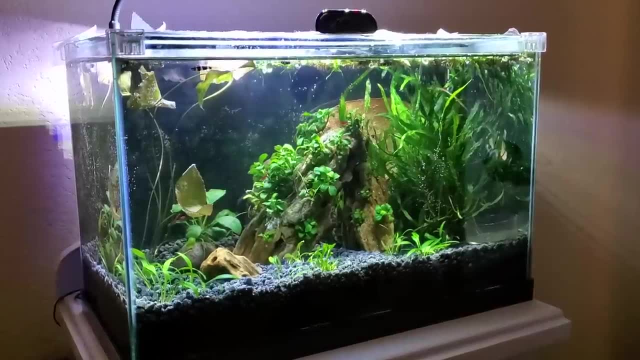 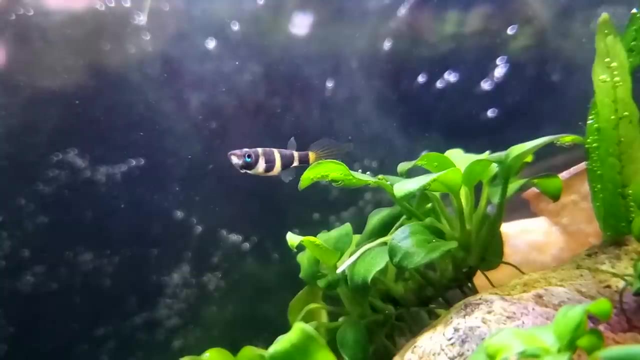 At this point. I am sick of doing that. That is not the life for me. As for how the five gallon tank is doing, this is around the time. I basically had one month of being out of commission for a medical emergency And I did not do any water changes on this at times.